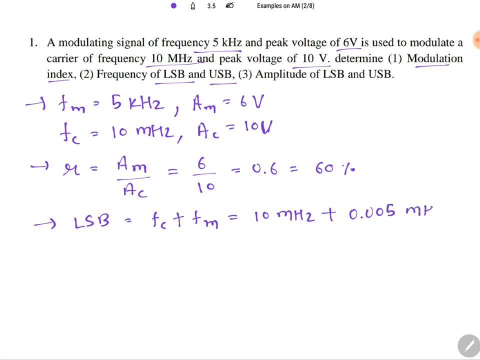 be 0.005 megahertz, So this frequency will be 0.005 megahertz. So this frequency will be 10 point. double. sorry, it is USB upper sideband, that is fc plus fm, So that will be 10.005 megahertz. 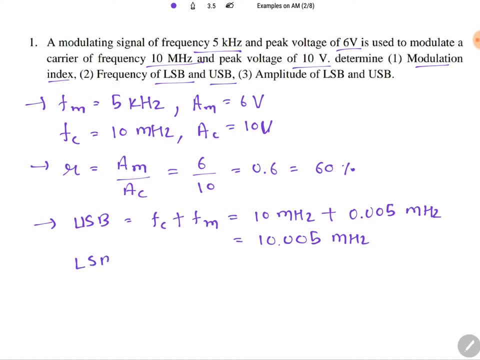 and for LSB it will be fc minus fm, So that is 10 megahertz, which is fc minus fm, that is 5 kilohertz and in terms of megahertz it will be 0.005 megahertz, So that frequency. 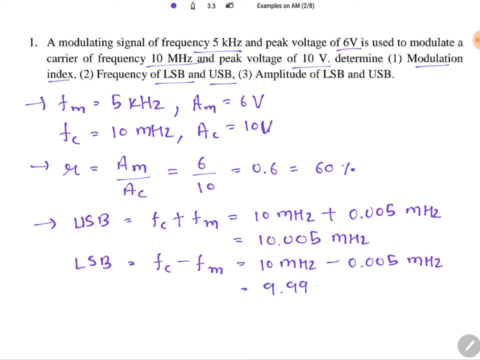 will be 9.995 megahertz. Now next question is: identify amplitude of LSB and USB. So amplitude of LSB and USB, that is mu, AC by 2, or one can say that is AM by 2.. So here AM is 6, so 6 by 2. 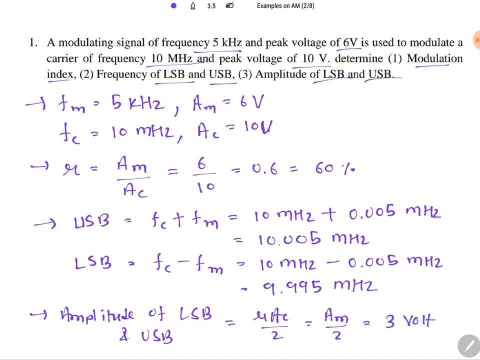 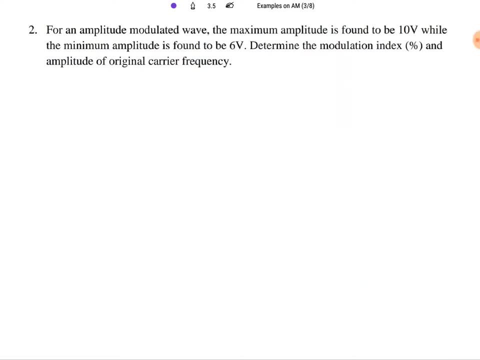 that is 3 voltage. So this is how we can identify basic parameters of amplitude modulated signal. Let us solve few more examples. So here in this question, for an amplitude modulated wave, maximum amplitude is found to be ten voltage and minimum amplitude that is. 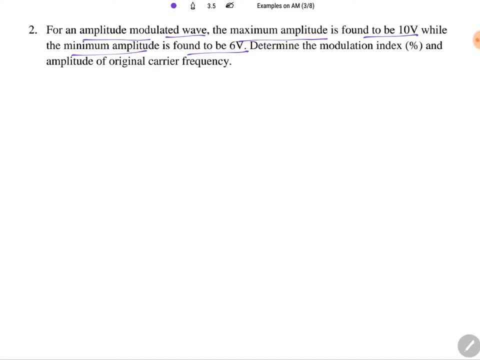 found to be 6 voltage. Then determine modulation index in terms of percentage and amplitude of carrier frequency. So here maximum amplitude, A max, that is 10 voltage, and minimum amplitude that is found to be 6 voltage. So maximum amplitude that is AC plus AM, where AC 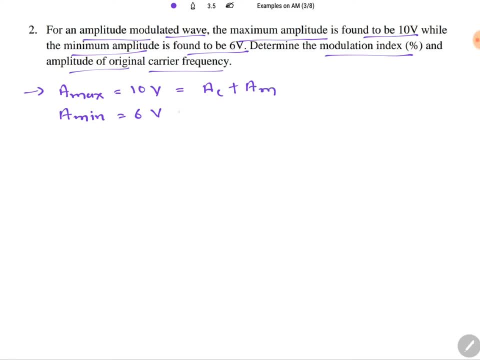 is carrier amplitude and AM is modulating signals- amplitude and A min. that is AC minus AM. So from that we can identify AC and AM. If you add this to signal then this AM will get cancelled. So this will be 2 AC and this will be 16.. So 16 is equals to 2 AC. So we can say AC is equals to 8 voltage. 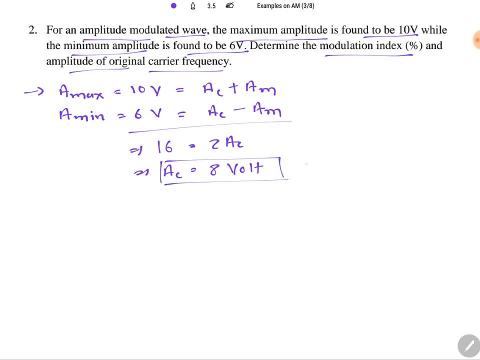 So now we have, AC is equals to 8 voltage. Now from this we can identify AM, that is, modulating signals amplitude, and that is 10 minus 8. So that will be 2 voltage. So AM is equals to 2 voltage. 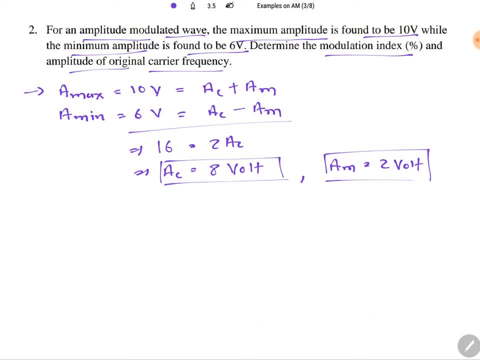 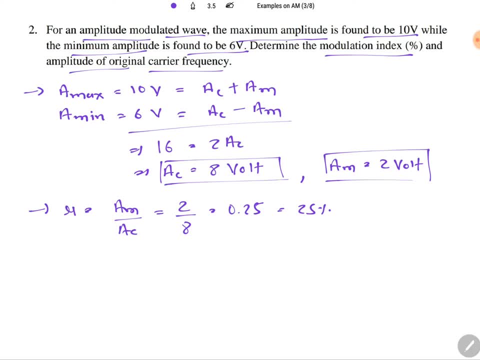 0.25, that be 25.. So 5 will be 25, and the amplitude of carry signal that we have already calculated, that is 8 voltage. So that is how we can solve problems based on amplitude modulation. Let us solve few more problems. 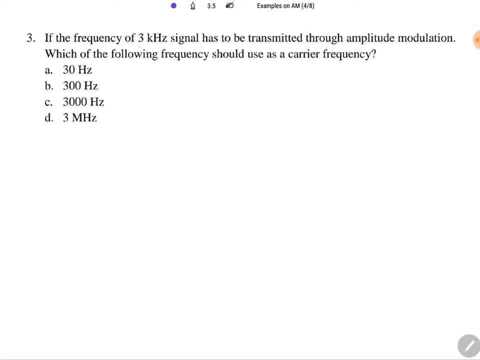 So here in this problem, if the frequency of three kilohertz is transmitted through amplitude modulation, Which of the following frequencies should be used as a carrier frequency? now, see modulating signal frequency. fm, that is 3 kilohertz, so obviously carrier frequency that. 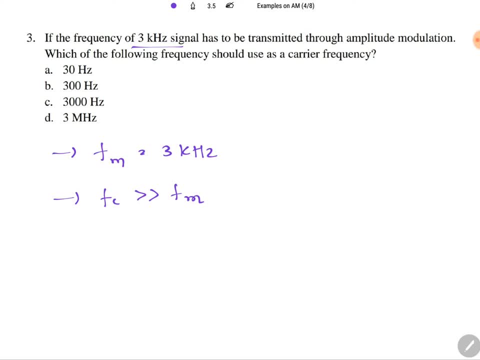 should be very greater than modulating frequency. so if you see first option, 30 hertz, so that is not satisfying our condition, so we cannot send it. 300 hertz, that is even lower than fc, so we cannot use it. and here 300, 3000 hertz, so that is what exactly equals to modulating signal. so that is. 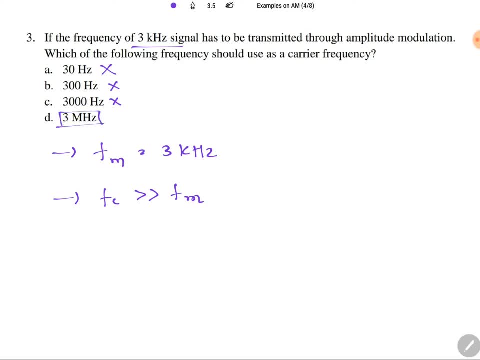 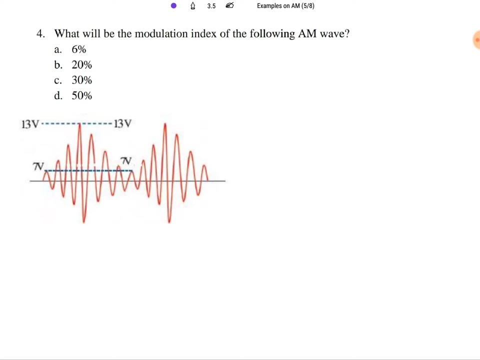 even we cannot use so 3 megahertz. that should be the case, which we should use it to send signal by amplitude modulation. let us solve few more problems over here in this question: what will be the modulating modulation index for given am wave? so here in this given am wave, maximum amplitude amx that we can see, that is 13 voltage. 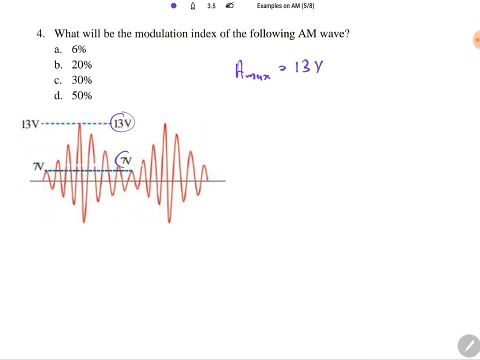 and minimum amplitude, that is 7 voltage. so amin, that is 7 voltage. now here amx means ac plus am and amin means ac minus am. now to solve this: ac and am. if you add this two, then this will result into 13 plus 7, that is 20, and this will be 2 ac and am will get cancelled. so from this we can say: 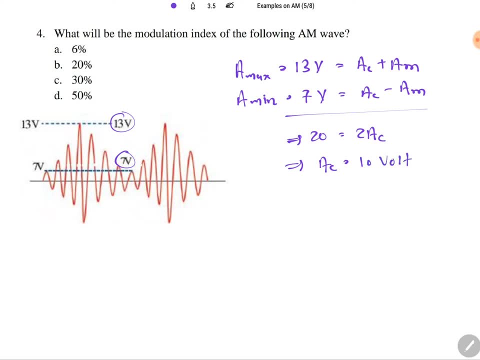 ac, that is 10 voltage. now we have ac is equals to 10 voltage. if you subtract in this equation then you will be having am. that is 13 minus 10, so that will be 3 volt. so from this we can say modulating index. so that is mu, that is. 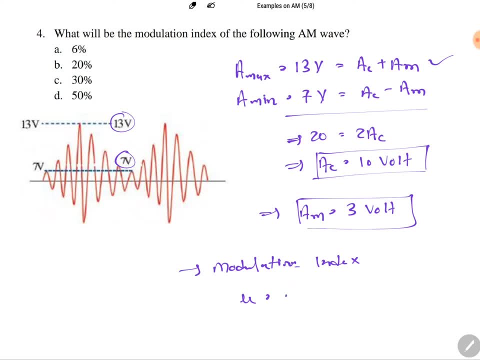 is AM by AC, and AM is 3 voltage, AC is 10 voltage, so 3 by 10, that is 0.3, means 30 percentage. So based on graph even we can identify what is the modulating index in AM wave. Now let us solve few more problems. 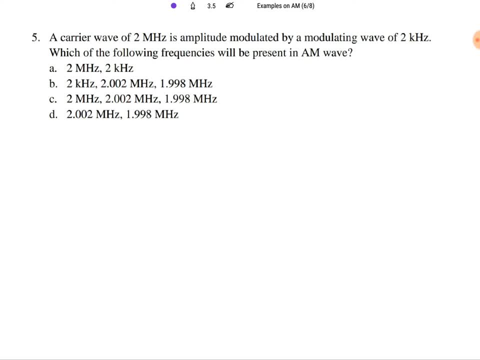 Now see in this question: a carrier wave of 2 megahertz is ambulator, modulated by modulating wave of 2 kilohertz, which of the frequency will be there in AM. So in AM wave there are three frequencies: one is fc, second is fc minus fm and third, 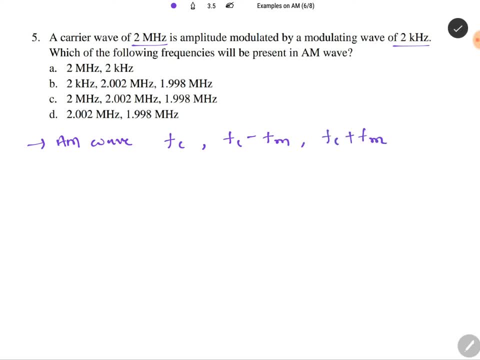 is fc minus fm. So in AM wave there are three frequencies: one is fc, second is fc minus fm and third is fc plus fm. So this three frequency component that is there in AM AM wave. So now here we have given with carrier signal with 2 megahertz, so fc that is 2 megahertz. 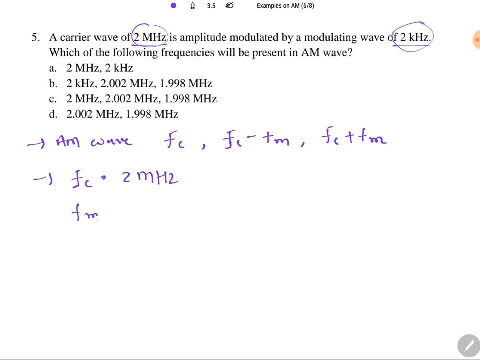 and modulating signal that is 2 kilohertz. So fc minus fm that is 2 kilohertz, it means that is 0.002 megahertz. so it will be having three frequency component. one is fc, so it will be having 2 megahertz component. this: 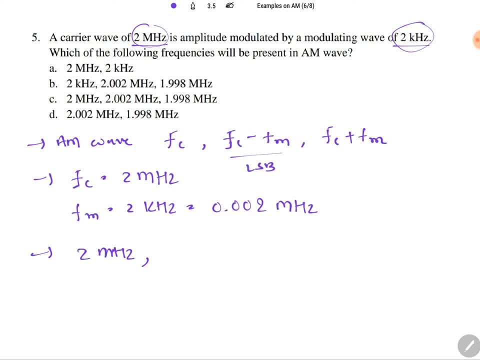 lower sideband, that will be fc minus fm, so that will be 2 minus 0.002, so that will be 1.998 megahertz, 2 megahertz and third component, that is usb frequency. that is 2 plus 0.002, so that will. 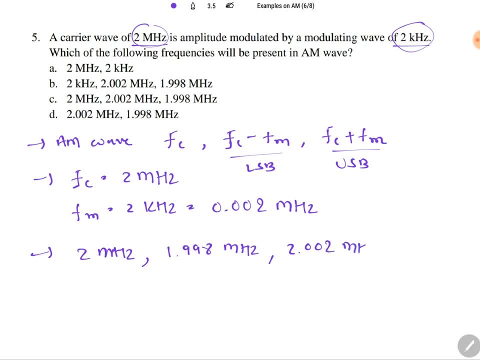 be 2.002 megahertz. So this three frequency component, that is, that will be there in AM wave. so our option should be this: 2 megahertz, 2.002 megahertz and 1.998 megahertz. 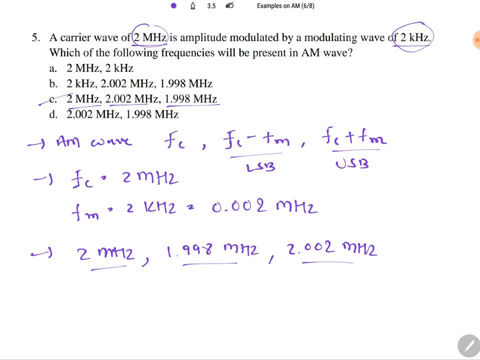 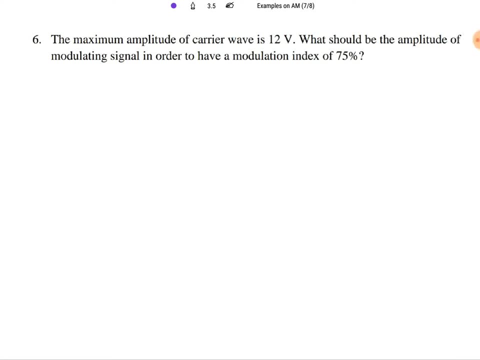 998 megahertz. now let us solve one more problem now here in this question: maximum amplitude of carrier wave, that is given by 12 voltage. what should be the modulating signal amplitude in order to have modulating index of 75 percentage? so here, carrier wave amplitude as ac, that is. 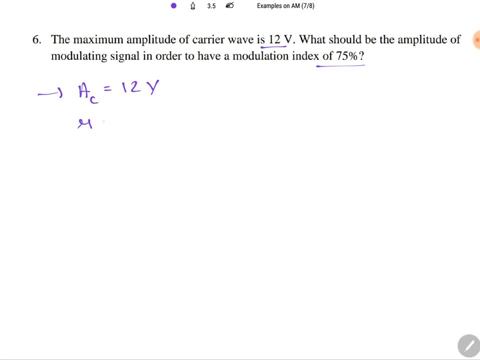 12. voltage and modulation. modulation index, that is 75, percentage means it is 0.75. now, as we know, modulating index, that is am divided by ac. so from that we can say: am, that is mu into ac, mu is 0.75, ac is 12, so 12. 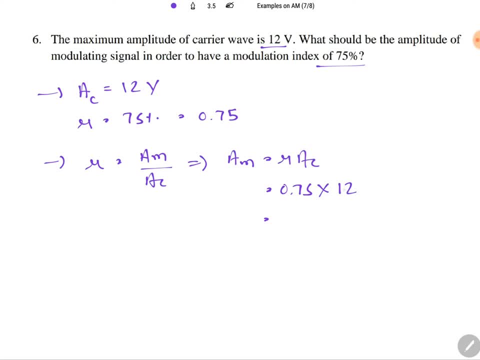 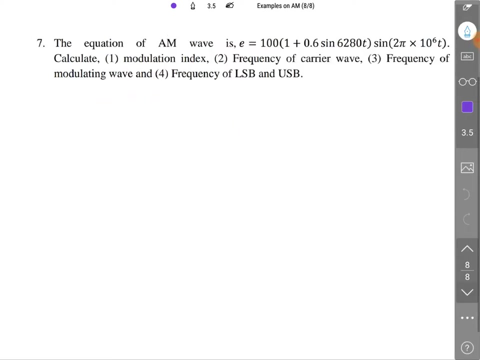 0.75 means 3 by 4 into 12, so 4 will get cancelled, 3 into 3, 9 voltage. so we can say modulating signal amplitude will be 9 voltage. now let us solve one more problem. so in this question equation of am wave that is given and that equation is: e is equals to: 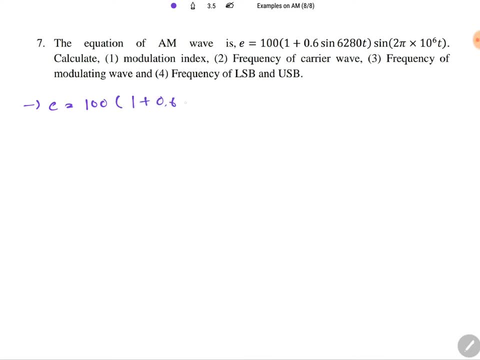 1 plus 0.6 sine 6 to 8, 0 t into sine 2 pi into 10 to the power, 6 t. so we are a little bit to calculate modulation index: frequency of carrier wave, frequency of modulating wave, lsb and usb. so 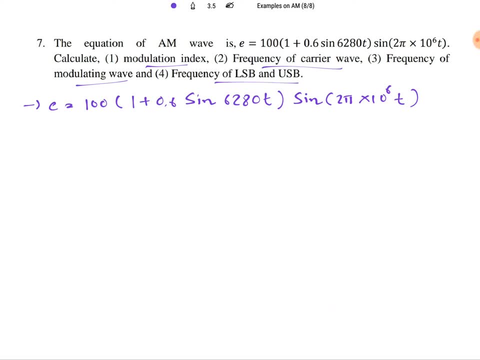 if you see my previous session of amplitude modulation, i have derived equation based on that and if you compare that, that equation was ac into 1 plus mu, into sine of omega mt, into sine of omega c t. so that is what i was explaining you in previous session. so if you compare this two, 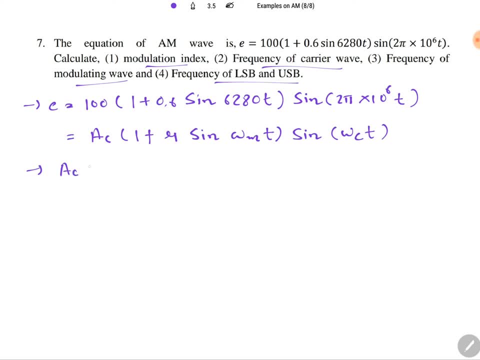 you will be having first parameter, that is ac, and that is 100 voltage. second parameter, that is mu, that is 0.6. now omega m, that is 2, 6, 2, 8, 0, so from that we can have fm, that is omega m divided by 2 pi. 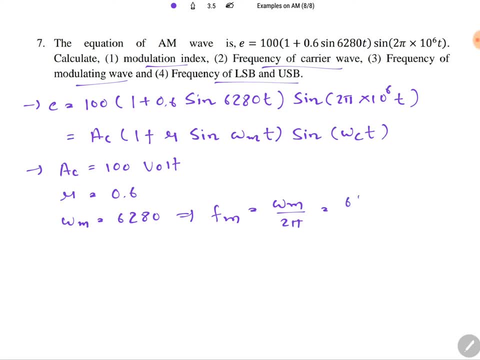 so that has to be 6, 2, 8, 0 divided by 2 pi, so that will be 1000 hertz. now next parameter: if you compare omega c, so that will be 2 pi into 10 to the power 6, so carrier frequency. that is omega c divided by 2 pi.